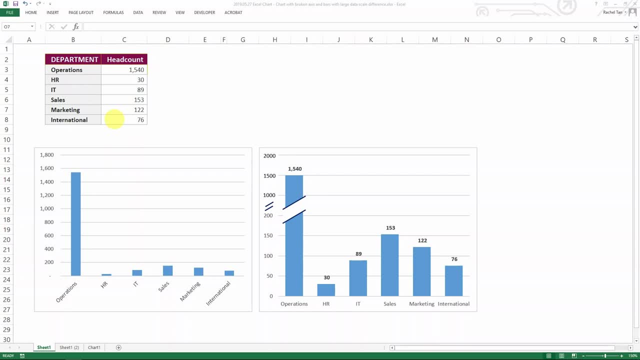 come across many cases where I find that I'm dealing with data with different skills, yet I have to show them on the same chart. So, for example, this is a very simple table showing the head count for different departments. but then this operation department has over 1,500 of employees, But then the other. 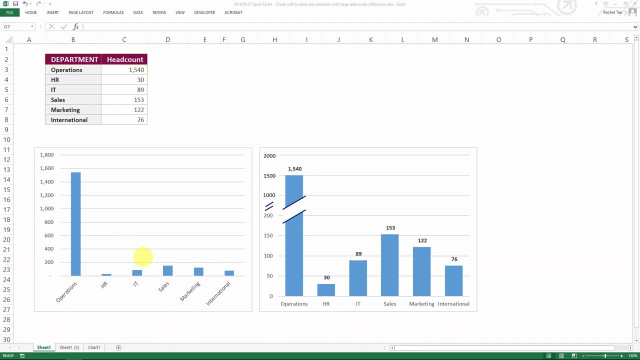 departments are showing relatively like small populations. So if we just show as it is, it doesn't really look nice, right? So it is much better if we just show them with: Yeah, OK, you get it. Alright, just getting ready, Make it quick. I mean, I see this. 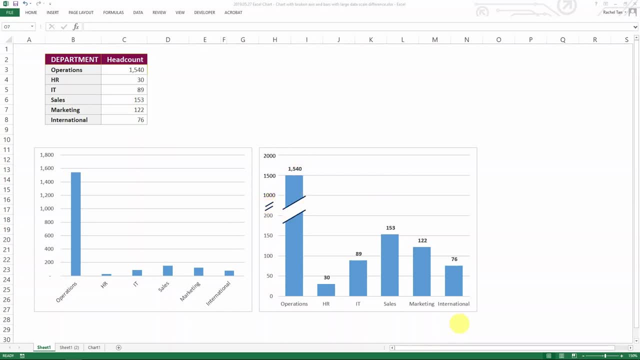 broken axis and bars here, so that they look much more pleasant compared to the one to the left. So I'm gonna show you two ways to do this. One is more easier and one is more simple, one is more complicated. So it's up to you which one. 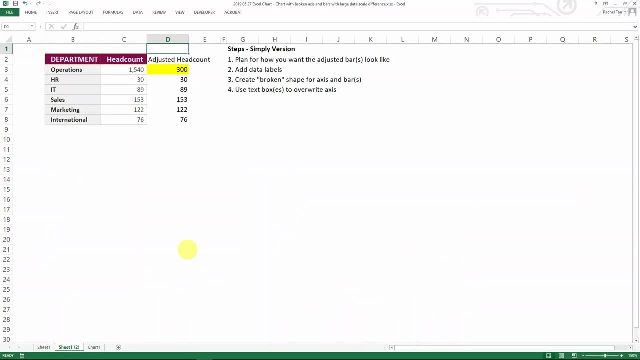 to use, depending on your case. So let's start with the simple method first. So let's do this, do the one without the scale first, so that's like an easy bar chart that we're looking at here, and then just let's just make it here as a 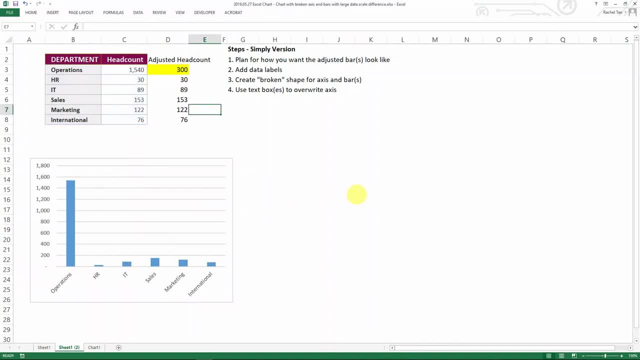 reference. And then, actually, the first step that we need to do is to plan how we want this bar look compared to the other ones. So to do that, actually, you can just copy the chart that we just did and then paste it to the raw. 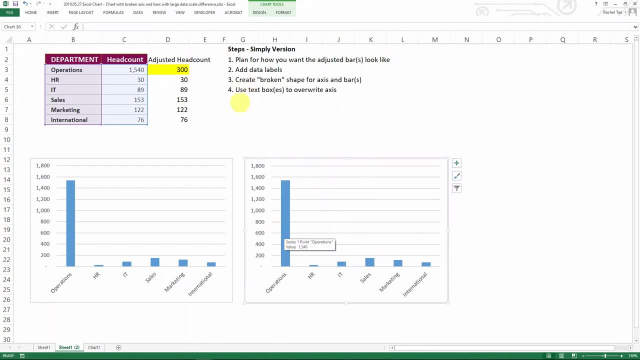 right, But then instead of having it referencing the headcount column, let's reference like: basically you have them selected and then you just move it to the adjusted headcount, which is a column that you're going to play out with. Alternatively, you can also do something. 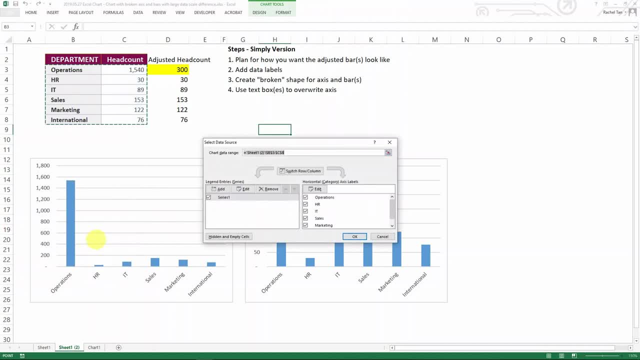 like selecting the bars that you have and then select data, go to Siri the data and then edit And then when you click in the Siri value, you see that it's referencing this column. Just actually make sure you have it clean and then select the adjusted headcount here. 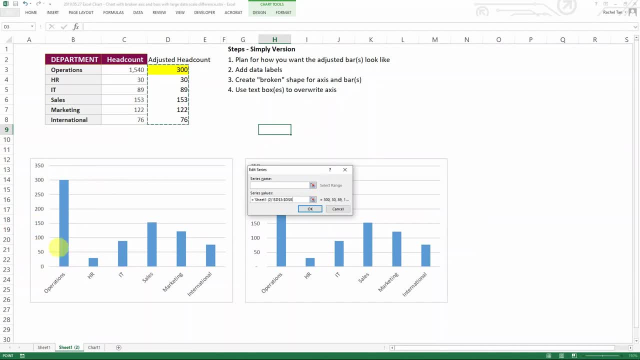 And then it's going to show it as the scale that we have here. So I'm just showing you alternative way to do it. So OK, so this is the scale that we have here. So I'm just: this is how it's looking like right now. So I've highlighted here as yellow, because this is the 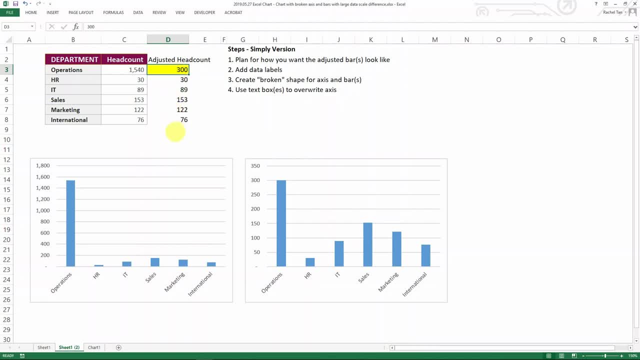 data that's so much more different than compared to the other ones. So the other ones are all below 200. But this one is like over a thousand, It's all. it's more than 50 times of the HR population. So it's. it will be up to you of how drastically different you want this bar to look compared to. 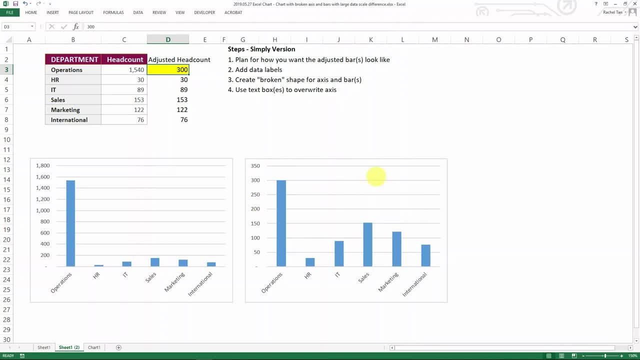 the other ones, For example, for 300,. this is how it's going to look roughly. But then let's say, if I wanted to look less dramatic, then you can put 200 and then you can see it's less dramatically different compared to the other ones. And you know what, if you want it to be even more, 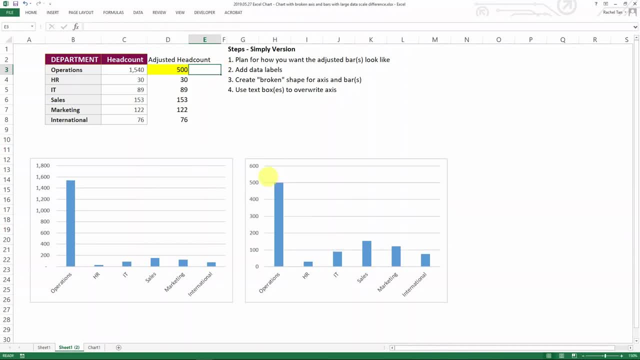 different. you put like 500, and then this one's going to look even larger compared to the other ones. So it's a. it's actually a just personal preference of how you want it to look. For me, I just decided to look around 300 there. Okay, so that's a scale I want to look. 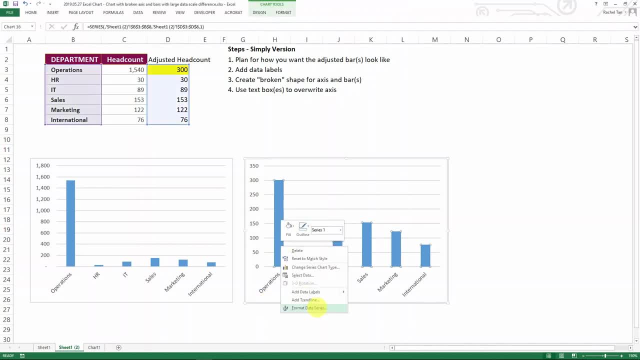 I want it to look like. And then basically I want to beautify my, my bars, So I always wanted to be wider. So to do that I go to gap worlds and I have it around 80. Like I just think I like. 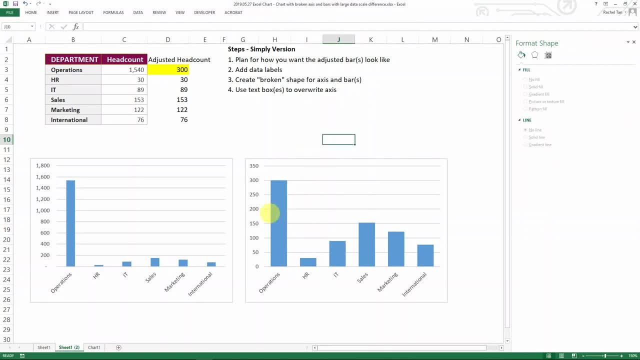 it better that way. Select your bars again and then right click add data label, And then you can see it's adding the label of the adjusted headcount that you you want And that is not the real headcount you want you. 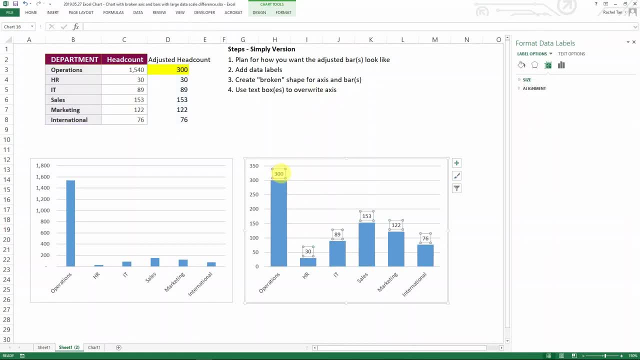 want it to show the real headcount right. So then what you do is select the data series, make sure every single data is selected, And then you go to format. It's selecting series, one data labels and a format selection, And then you can see on the right you have the label options. 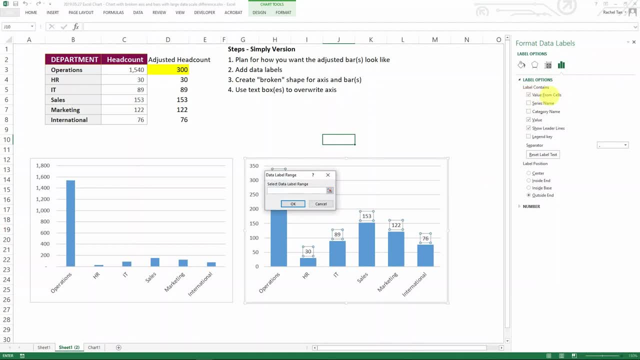 So for this you actually need to click value from cells which allow you to select the data label range, And then this is when you select the real headcount, like this, and then you go okay, and then it's gonna look like this, And this is because you have the value and show leader line selected. 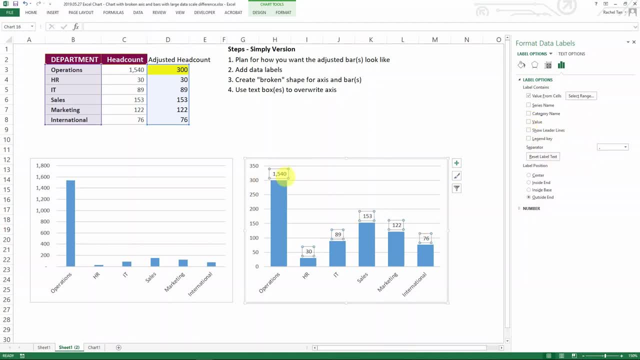 So you know what? just unselect it And then now it's showing the real headcount for you, And then you can make it like bold. I always make my data label bold, So it's 10.. ok, So now we have, we have the bars, and then we have the right data label. So let's create. 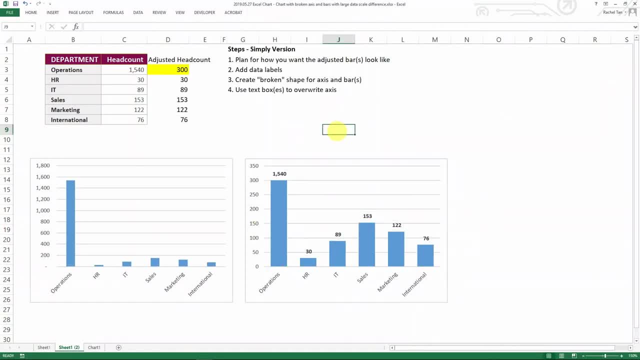 the break shape. So to do that, you can actually just do it by insert a shape like that, And then what you do is you go format: I want it to be filled with white or whatever color that's identical to the bar with the expected size, And these are gone. Okay, now this is what this Farm. 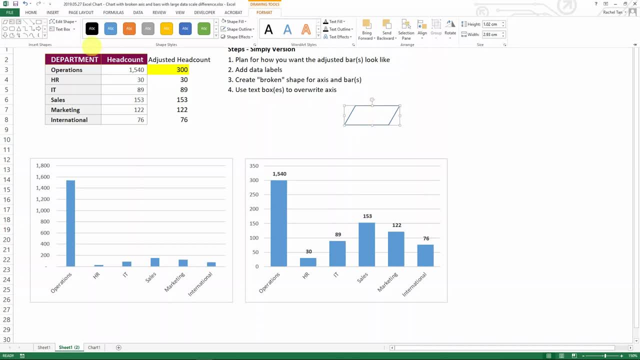 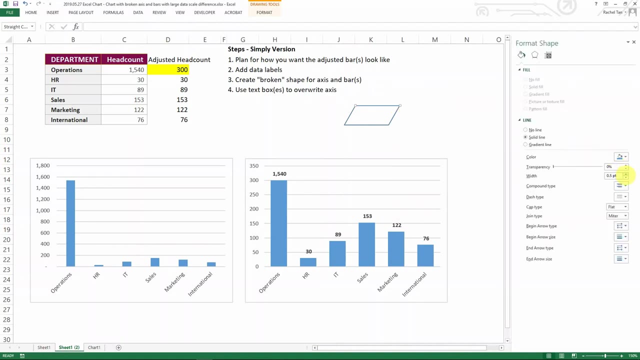 background of your chart, and this is now is how it's looking like, and I add a line to it to the top and the to the top and the bottom of the chart and you can see those two squares and then I go format my shape and then I want to change my line to some darker color and I want it. 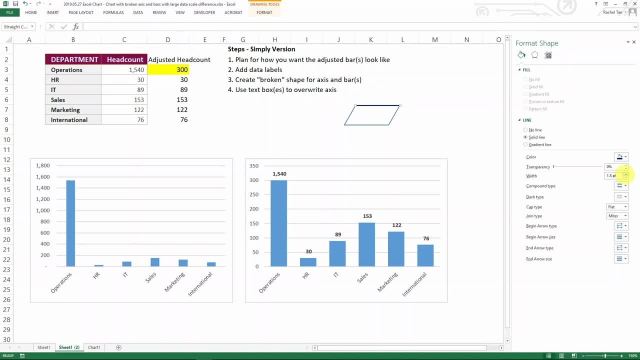 to be 1.5, so that you can see like it's actually thin, thicker. yeah, I want it to be a 1.75, and then I select this line, copy paste and then make sure I have it overlap the bottom as well. so now I have. 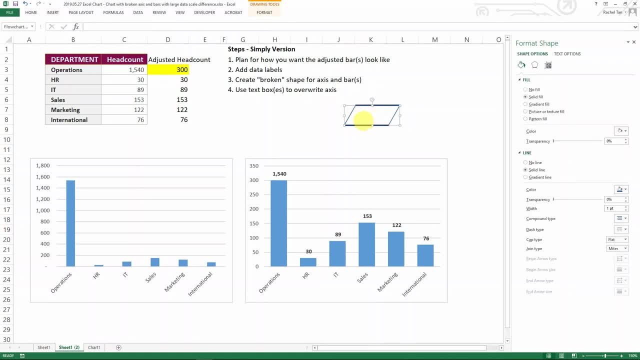 those two covered and I select the shape again and then I want to get rid of the outline, so I say no outline. so my shape basically look like this: so I have three parts. I have the two lines, you have control selected, and then you select the three parts and then right click group and then 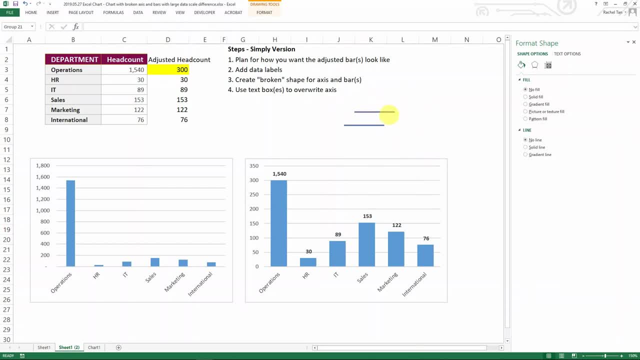 group. so that is the breakout shape that you're going to use for your, for both your- uh, your bar and your axis. so okay, so now let's move, like, reshape it to whatever that fits your bar, and then you want your bar to be a little bit slipier. so if we're having a halt over here, I want to. 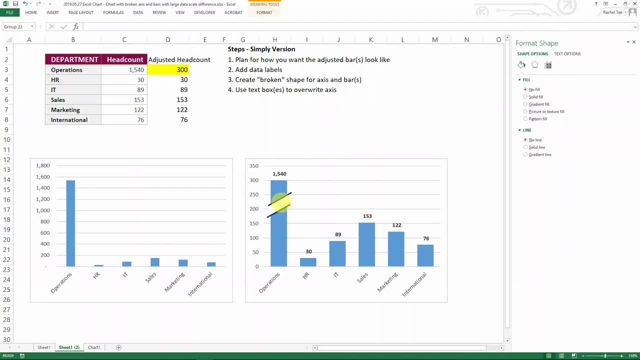 maybe change a position a little bit. I want it to be around like a approximately 45°, and I have it here, and then I just move it to wherever my bar is, and then you can just adjust the shape to whatever that's appropriate for you, and then here you go. so that's how it's looking like broke. 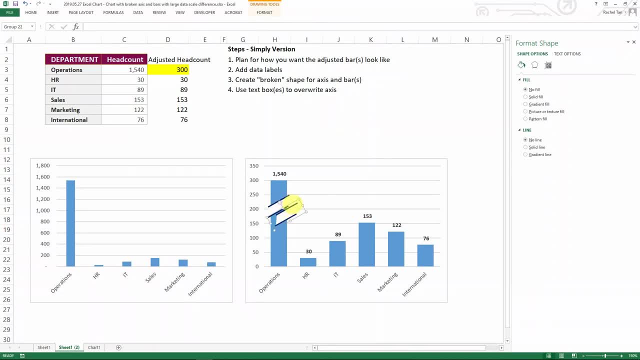 For you And then select the shape again, Copy paste, So you have another one. and then you just keep saying, oh, it's gonna be okay, and you go and your bar is all changed. so that's the first step, and if you're crossing your bar, you're just going to go down to fit the bottom view. right now, 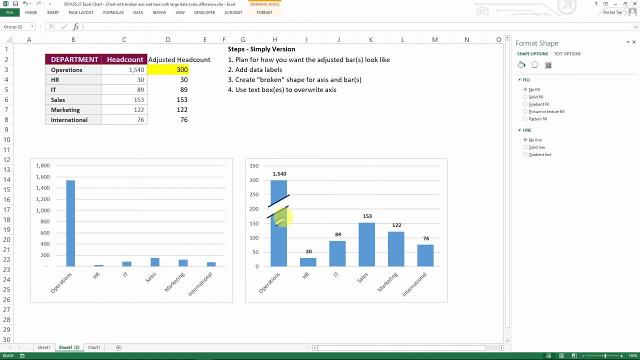 if you're taking all of those and then you link down, you're going to find each bar you see on the top. so if on top of those bar- that's the bottom view, so you select the left, Okay, just shake it, shrink a little bit and then put it across the axis, because 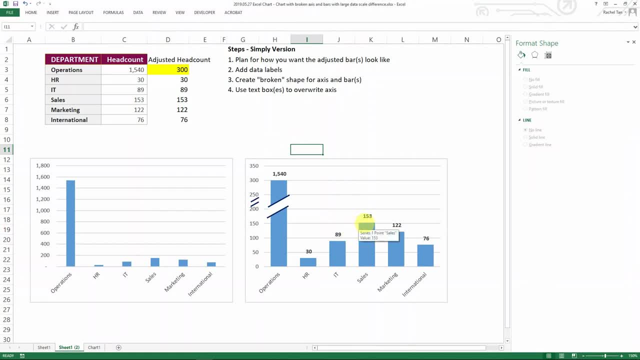 actually, you know what you can see like. we have a data of around 153, so we want the 153 still to be the same scale, 200 to be the same scale, but then for those three labels above we want it to be about a thousand. so there's a simple. 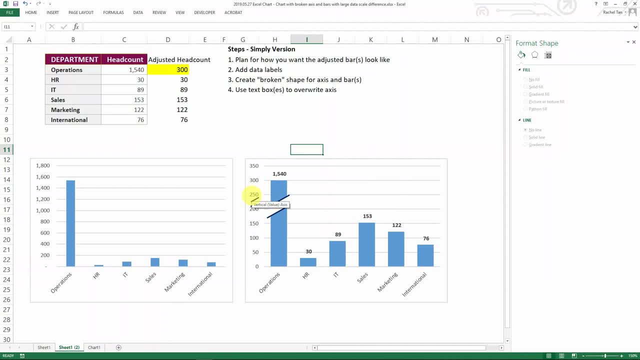 way to do this is actually just put text box into over this and overwrite it. but there's also another, more complicated way to do it, so let me do do it with the simple way first. so you insert a white box to cover the original text first, and 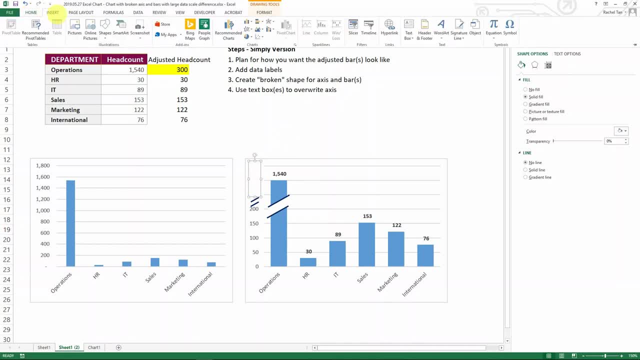 then you put in your text box- you know, actually text box, put a text box, make sure there's no background, no white background, no line. and then let's say you want it to be like a thousand, make sure it's the same size of text as your other axis. so I know it's Calibri.